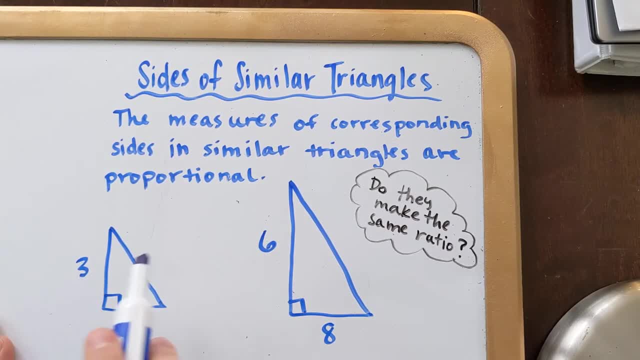 meaning we're going to divide them. And if, when we divide these two sides, if that makes the same number as when we divide these two sides, then it is similar. All right, let's take a look here. So I'm going to start with these corresponding sides: the 6 and the 3.. 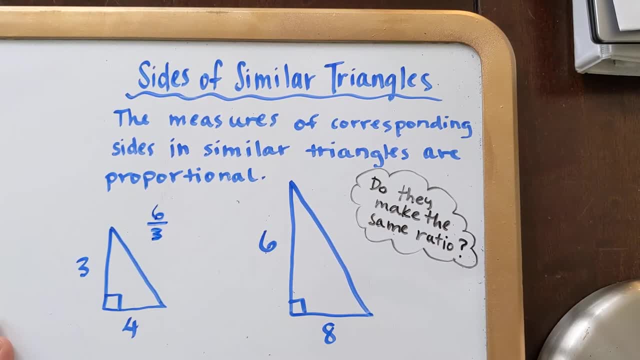 I'm going to divide them. I'm going to make a ratio. divide them 6 over 3.. All right, now I know that makes 2.. The question is: when I do the other sides, the other corresponding sides, do those also make 2?? 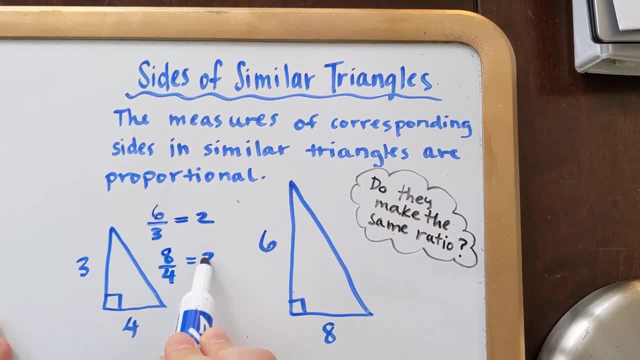 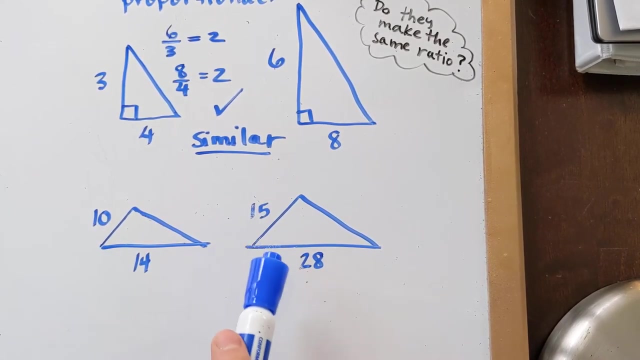 Well, let's see here: 8 divided by 4.. Yeah, definitely, So you would be able to conclude that these two triangles are similar. All right, let's try a different example here. Okay, so I can see I have a triangle here with a 10 and 14 and a 15 and 28.. 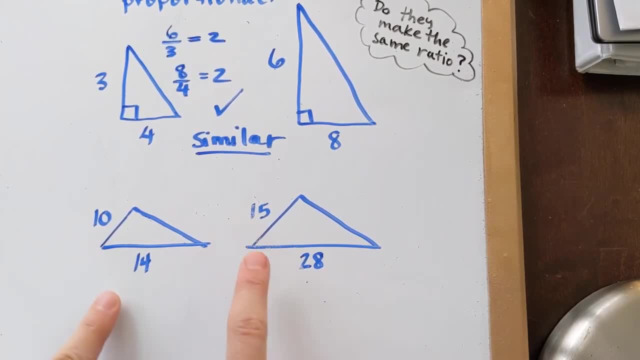 It looks to me like these are corresponding sides and those are corresponding sides, So we are going to divide them and figure out: do they make the same ratio? If you want to do it yourself, pause the video right now, Otherwise I'm going to go over it. 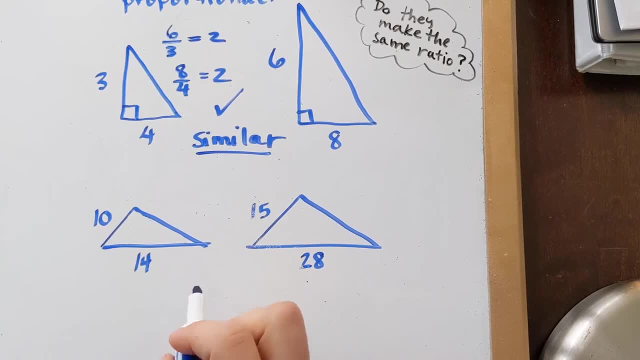 Okay, so I know that 15 and 10 are corresponding. They're in the same position relative to these triangles. So 15 divided by 10. When I do that, I get 1 and a half. So we're hoping that the 14 and 28 also make 1 and a half. 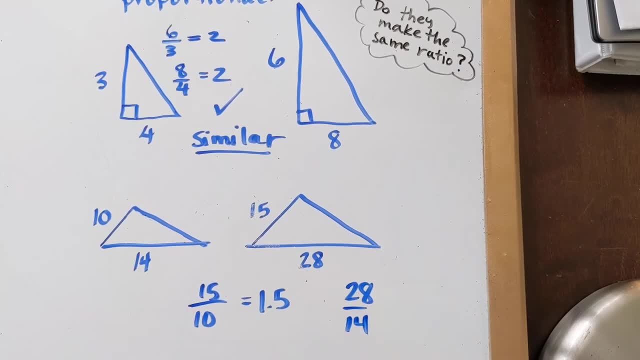 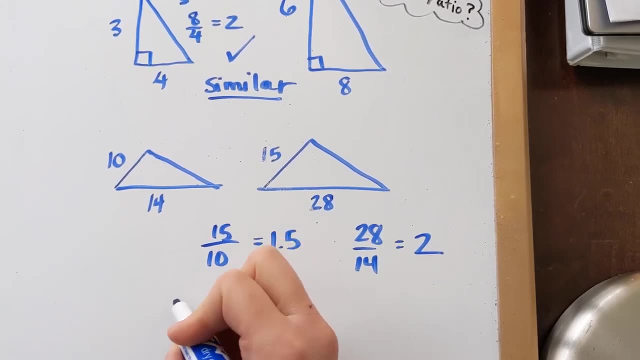 Let's try it out: 28 divided by 14. When you plug that into your calculator, actually you get 2.. So these two triangles are not similar, Not similar. Okay, a little bit of a different example going on here. 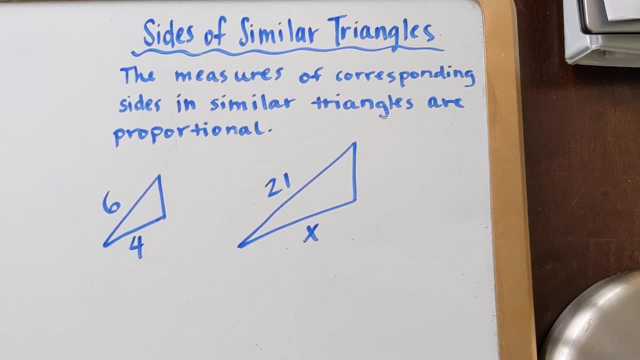 So we found out before that if you're given the side lengths and you're trying to figure out if two triangles are similar, you can do that by using the ratios. But if you're told already that two triangles are similar, then you can actually use that, use the ratios to find out a missing side. 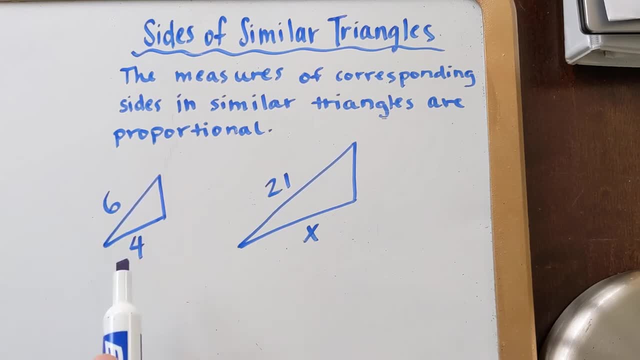 And so in this example here, let's assume we've been told that these two triangles are similar And we want to know what this side length is here. Well, we can use the ratios that we have, based on the corresponding sides, and we can figure it out. 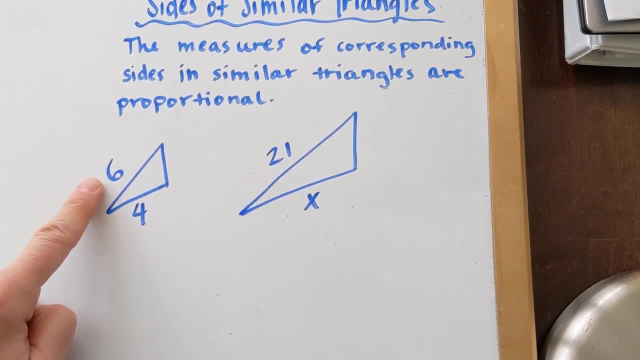 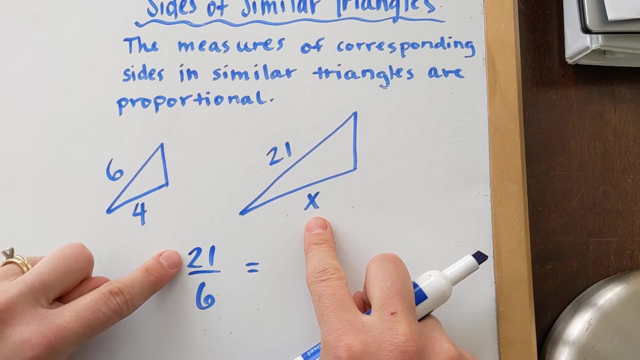 So let's take a look here. 21 and 6 are corresponding. So I'm going to just set up that ratio: 21 divided by 6. And I'm going to set it equal to the ratio here Now, because I started with 21 in this ratio. 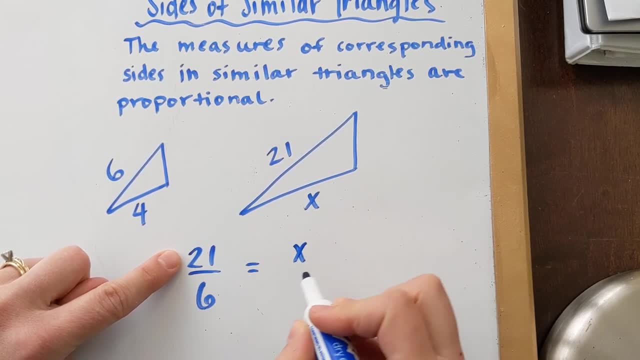 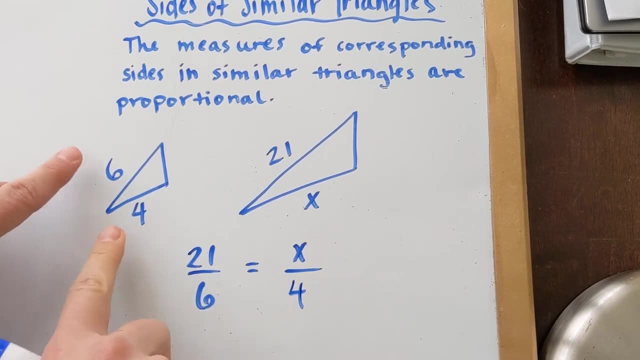 I also want to start. I'm going to start with X on the other ratio. all right, So it looks like the numerators are coming from this triangle and the denominators are going to be coming from this triangle. Just make sure that you're going in the same order when you do that. 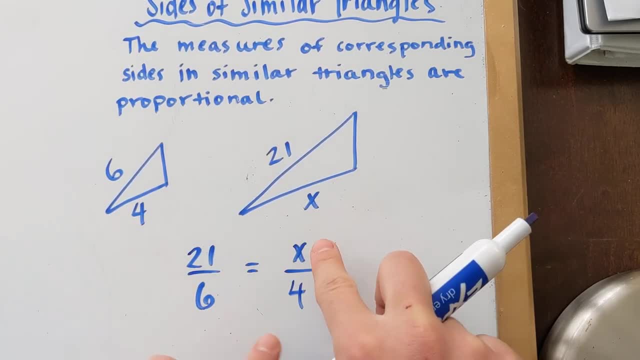 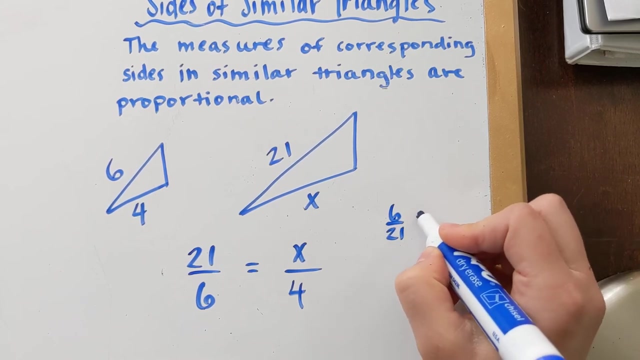 So corresponding sides, corresponding sides, but also keep that second triangle on the top and this triangle on the bottom. It would also be okay if you wanted to use um. 6 over 21 equals 4 over X. Just make sure again, like I said, it goes in the same order. 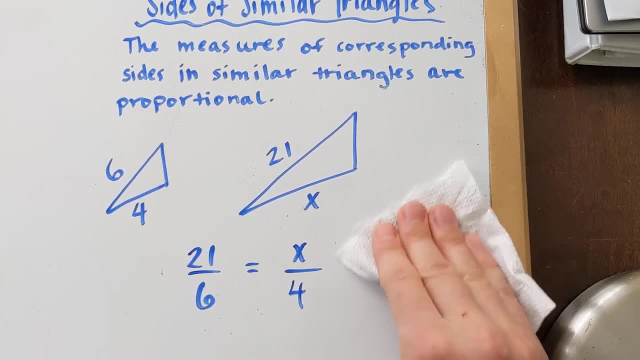 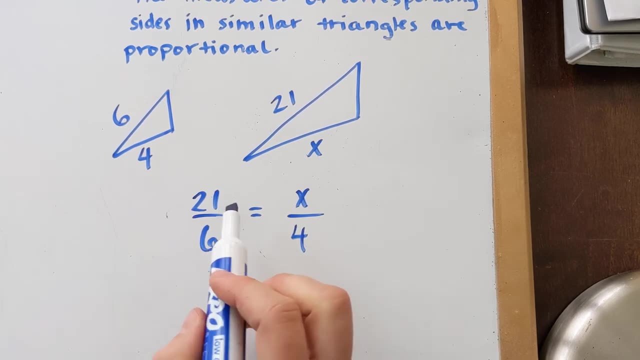 So triangle 1, triangle 2.. Okay, When you are solving a proportion, you do that by cross-multiplication. So I am going to be multiplying the 21 and the 4.. I'm also going to multiply 6 and X. 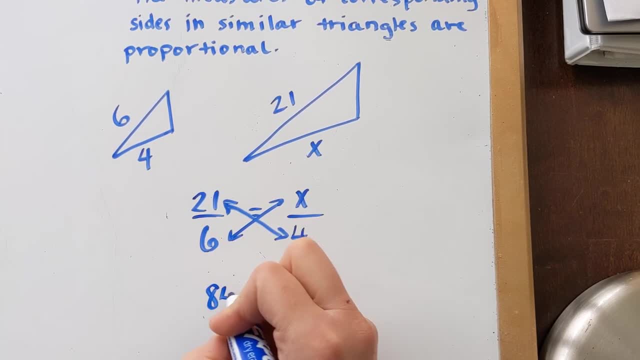 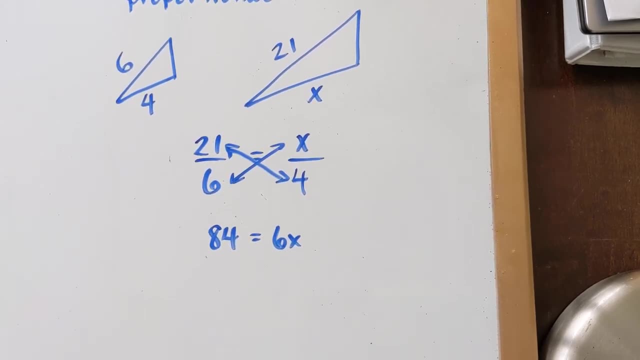 So 21 times 4,, I'm going to get 80.. I'm also going to multiply 6 and X: I'm going to get 4.. 6 times X, I'm going to get 6X, And then all I would be left um doing is dividing by 6.. 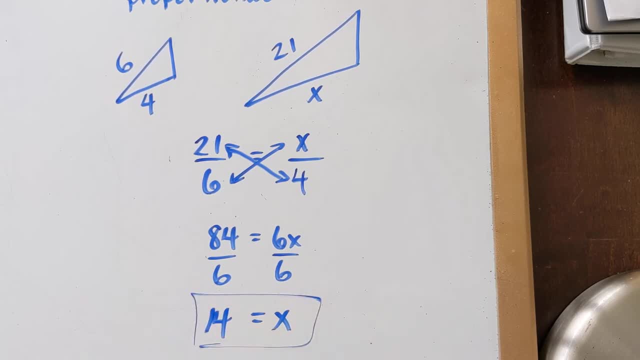 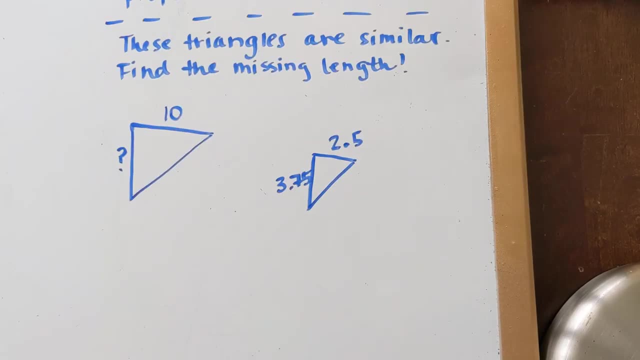 And I would get X equals 14.. So that missing side length there is 14 units. I'm going to have one more example and I want you to try it without me. Okay, here's your example. I have two triangles. 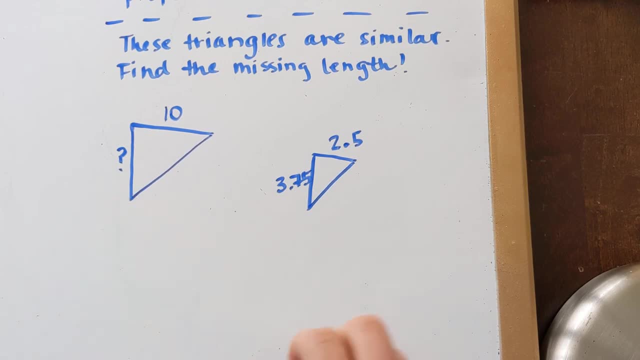 I'm told that they're similar. The length is right here. This side is 2 1⁄2, this side is 3 3⁄4.. I have a side of 10, and that's my missing side.